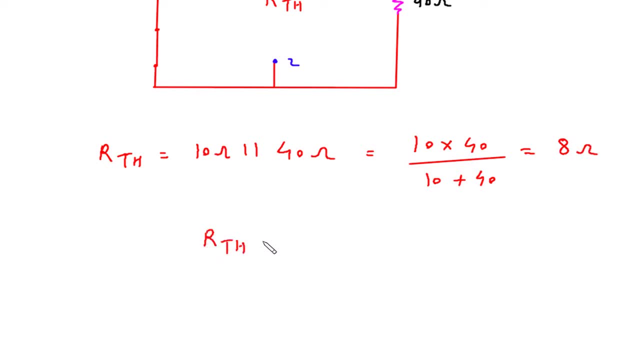 Therefore, Rth is equal to 8 Ohm. Next we have to find Vth. So to find Vth, To find Vth, This will be Vth. Let's say this is node V1.. And this is ground. Let's say this is current I1.. 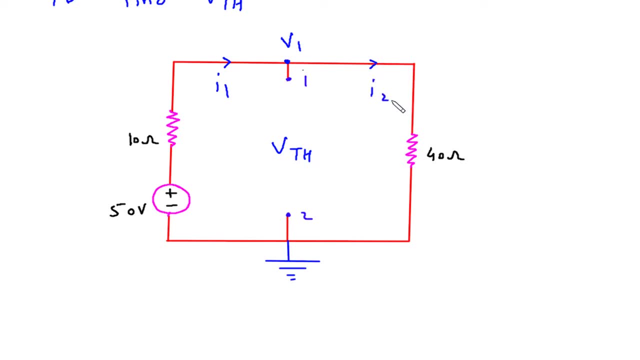 And this is current I2.. So here we can apply KCL. Apply KCL at node V1.. So summation of all the entering current: Entering current is I1 and leaving current is I2.. So I1 is equal to I2.. 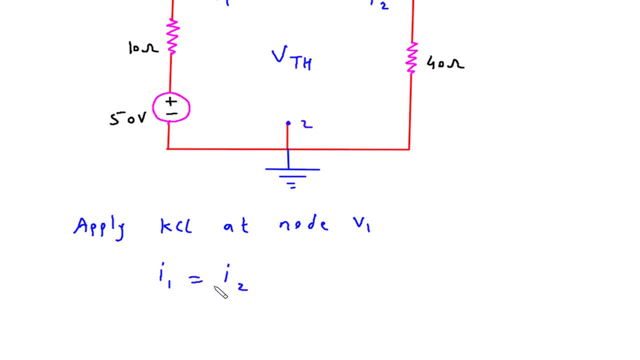 I1 is equal to I2.. Now I1 is I1 is 50 minus V1 by 10.. 50 minus V1 by 10 is equal to I2.. I2 is V1 minus 0 by 40.. 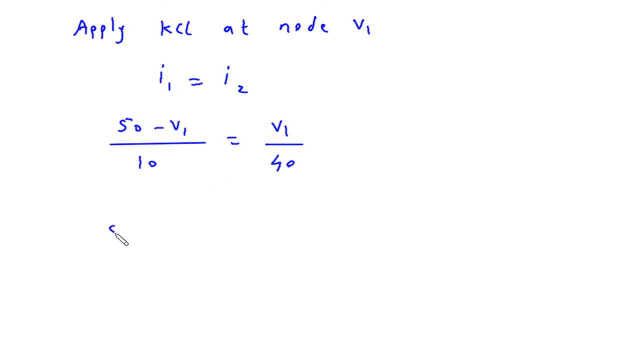 V1 minus 0 by 40. So this will be 50 by 10.. Minus V1 by 10. Minus V1 by 40 is equal to 0. So this will be 5.. And this will be minus 1 by 10.. 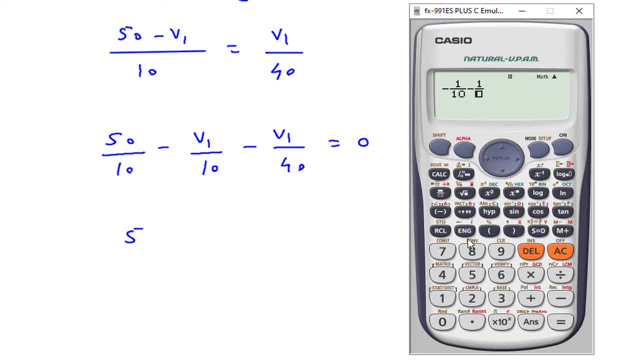 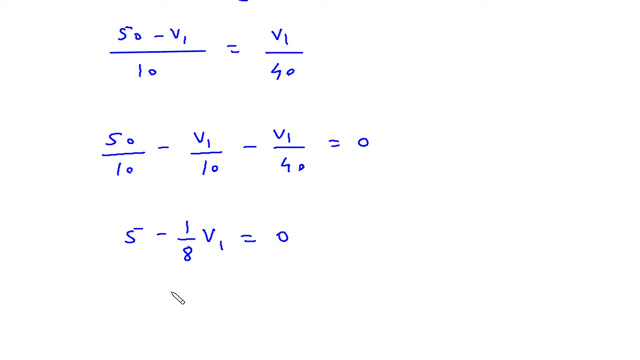 Minus 1 by 40.. Minus 1 by 8, V1 is equal to 0.. So 1 by 8, V1 is equal to 5.. Therefore, V1 is equal to 5 into 8.. So this will be: V1 is equal to 40 volt. 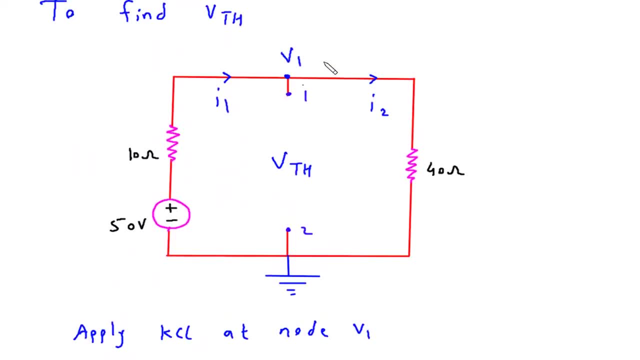 Now, V1 is equal to V1 is equal to Vth, V1 is equal to Vth. Therefore, Vth is equal to 40 volt. We have the value of Rth and Vth. From this we can draw the Thevenin equivalent circuit. 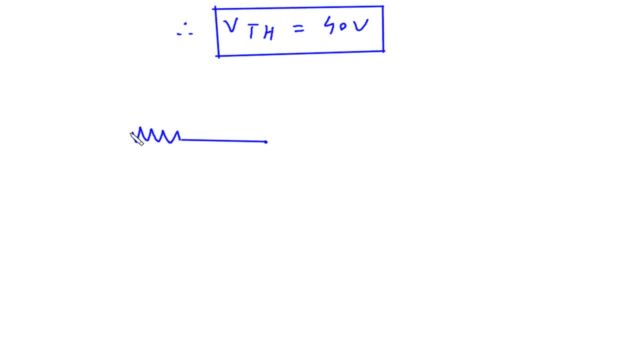 So this will be Thevenin resistor, Rth, Rth, And this is Thevenin voltage, Vth. This will be plus, This will be minus. This is Vth. Vth is equal to 40 volt And Rth is equal to. 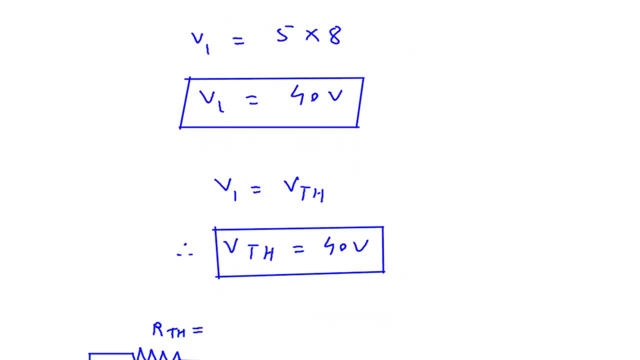 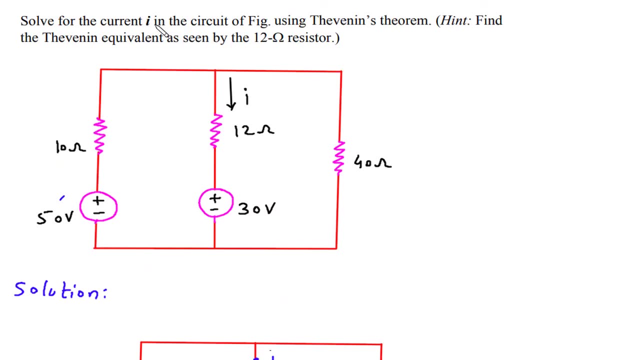 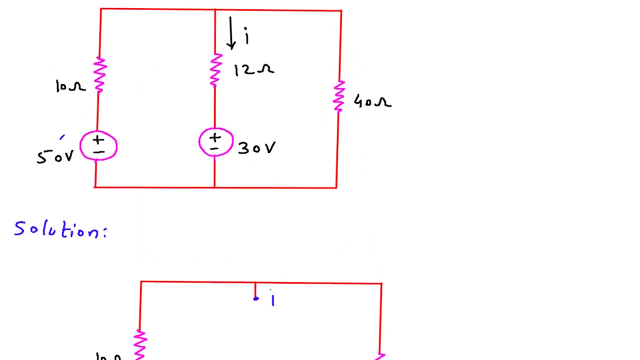 Rth is equal to 8 Ohm- 8 Ohm. What we have to find? We have to find current I, using Thevenin's theorem. We have to find this current I. Now we have replaced this with Vth and Rth. 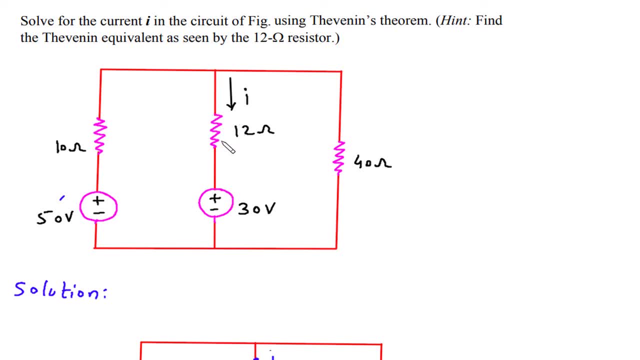 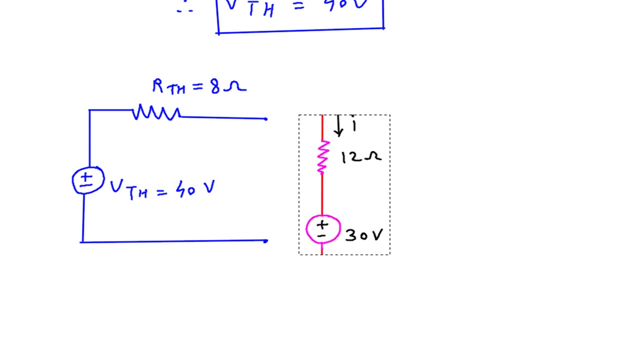 Now we will put it back, So 12 Ohm in series with 30 volt. So we will connect it here like this: Now, here we can apply KVL. Let's say this is current I And we will start from here. 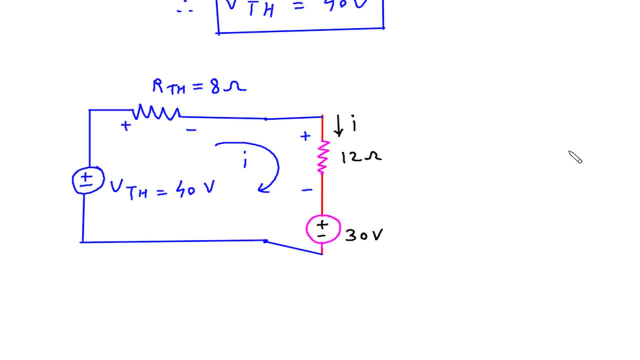 So this will be positive. This will be negative. Positive, Negative. So this will be minus 40.. Minus 40. Then this will be 8 plus 12 will be 20.. So plus 20 I 20, I plus 30 is equal to 0.. 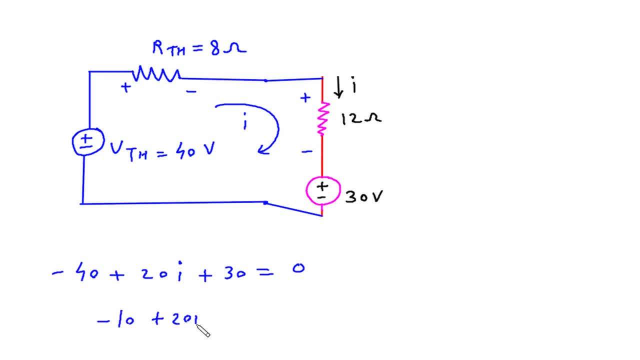 Now this will be: minus 10 plus 20, I is equal to 0.. Minus 10 plus 20, I is equal to 0.. Now this will be 20: I is equal to 10.. Therefore, I is equal to 10 by 20.. 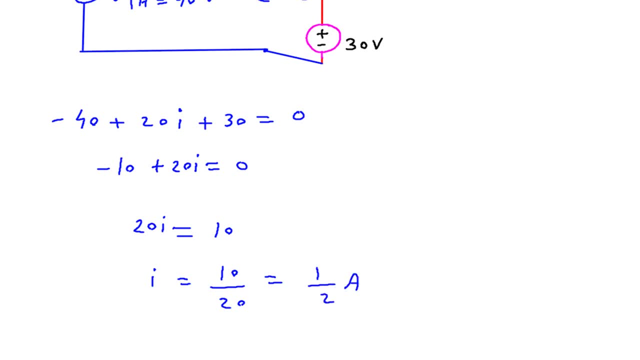 So this is equal to 1 by 2 Ampere. Therefore I is equal to 0.5 Ampere. For Electrical and Electronics Engineering related questions and answers, visit the link in the description below.